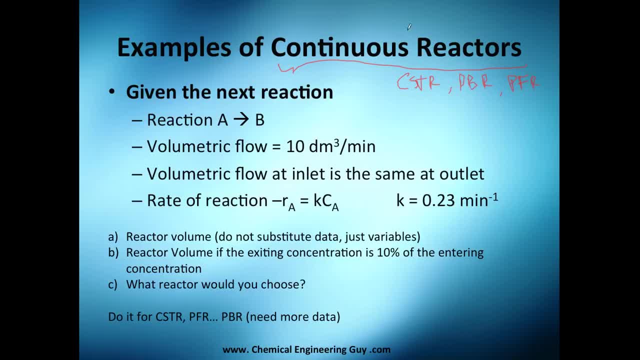 plug flow reactor and back bed reactors are continuous. Batch reactor is not a continuous reactor. So they tell you, given the next reaction you got, A transforms into B, you've got this volumetric flow rate which is essentially 10 cubic decimeters per minute. You know that the volumetric flow 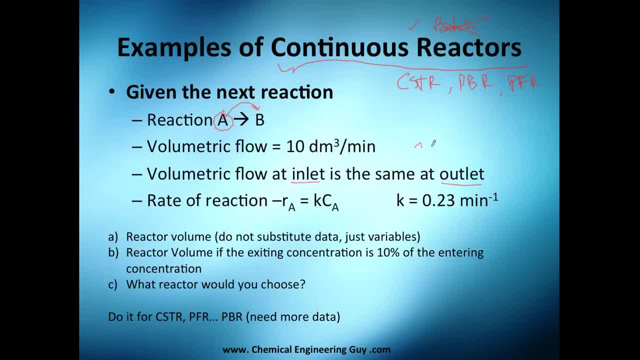 rate at the inlet is the same as the outlet. so let's say this is constant. and they give you the rate of reaction, which is essentially not a value but it's dependent on concentration. so you got this K, which is a constant 0.23 minutes, and this concentration, so it 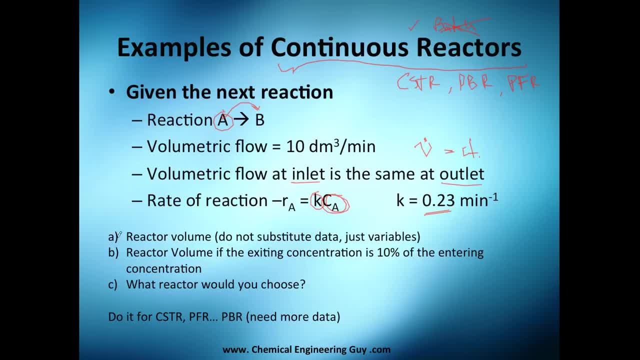 varies with concentration. They tell you number or letter A. please give us the reactor volume and do not substitute data, just variables. Okay, so once we got that, if the exiting concentration is 10% of the entering concentration, what? what? I think you're going to calculate the volume here and then they tell you what. 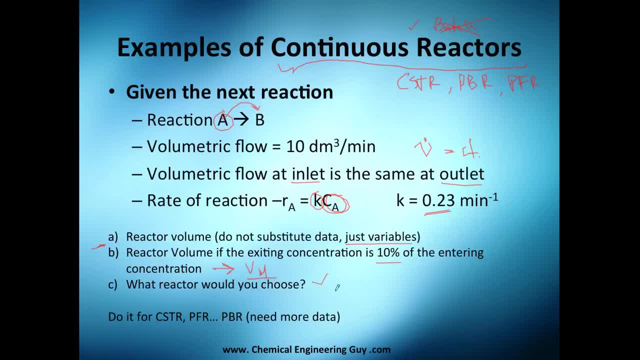 reactor would you choose? So we're going to do it for CSTR continuous shear tank reactor and plug flow reactor PBR. no, Why not? Because we will need more data, more about the mass reactions these reactorsapped that one down. Roxanna saidover they trust us. they're going to remember this. 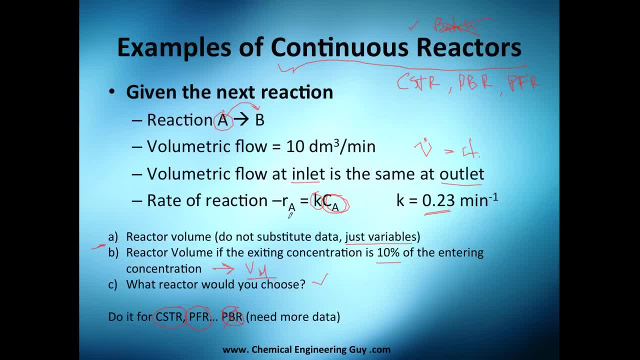 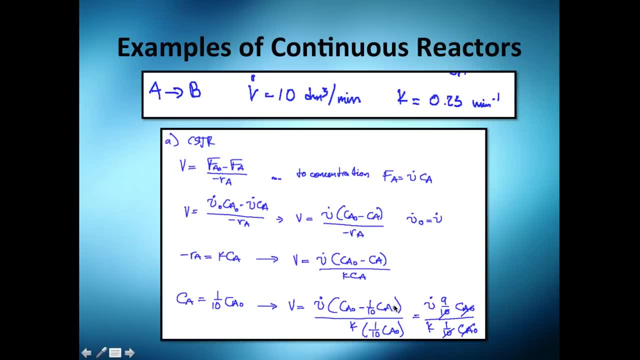 about the constant or the rate of reaction. we will need this prima and essentially only CSTR and PFR. so I got this data: the reaction, the volumetric flow rate and this constant. okay, let's do it first for the continuous tier tank. so I got this my master equation. let's change it to concentration. we could. 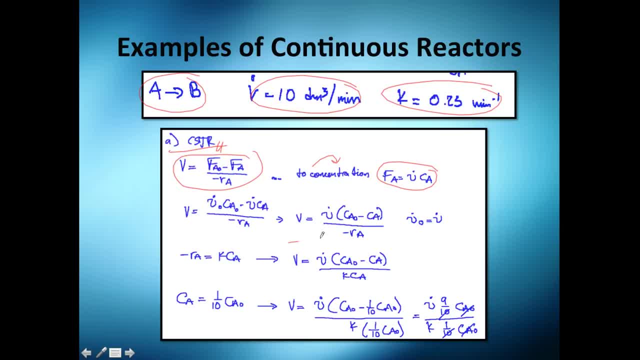 either go directly and look out for this. this is my equation, but I'm just going to do it so you can see that you can actually do it every time you want it. you don't need to go directly to your formulary. if you know this very well, you can change it. we just remember Flows and 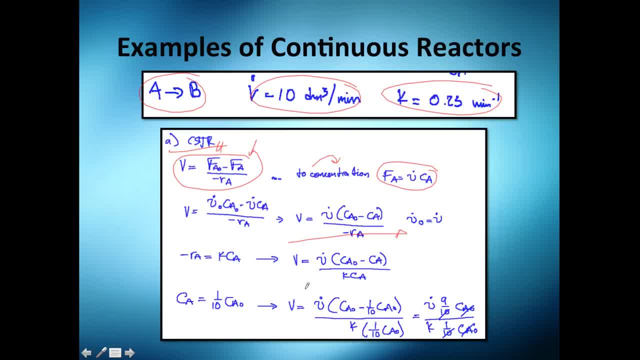 concentration have a relationship and yeah, let's just substitute- this will be my question. and now let's just do the rate of reaction, which is k times concentration, which is here. I just substitute this here. and they tell me they wanted the final concentration. they want it to be 10% of the initial concentration. 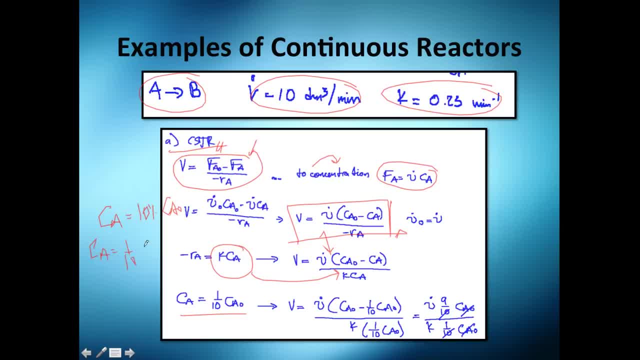 how do we do that? It's essentially one tenth of that initial concentration which is here. okay, so let me just substitute that. so I got this initial concentration. that stays the same minus the final concentration, but the final concentration is one tenth of that initial concentration. so I got this and 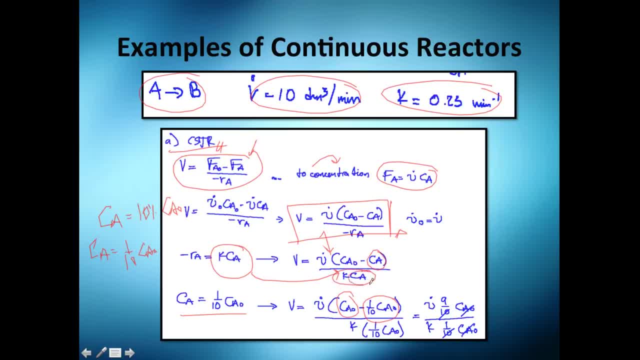 this concentration is also final, very important. it's not the initial, it's the final concentration. so let me once again substitute one tenth of the initial concentration. now, as you can see, this will get 9 times divided by 10,. volumetric flow rate stays there. initial concentration stays there. 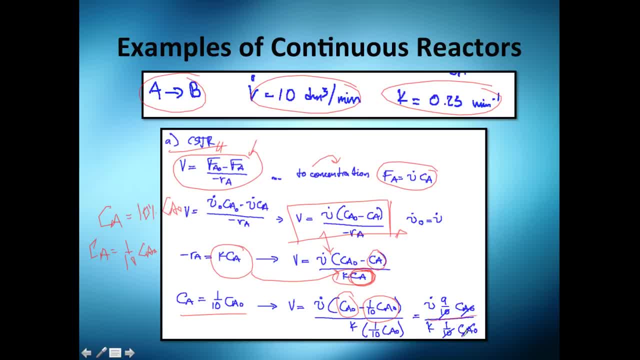 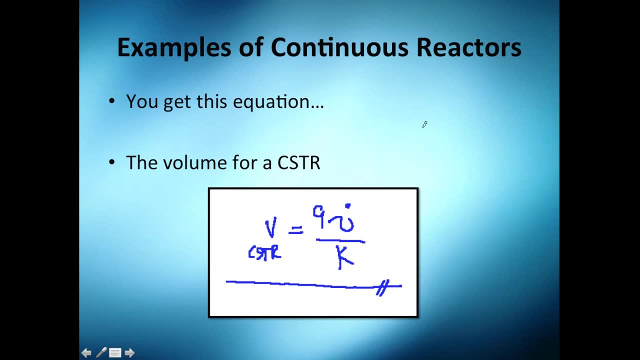 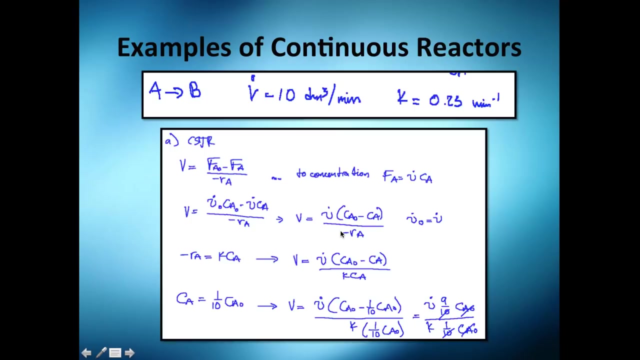 all this divided by k times one tenth times concentration in the initial state. so this is just algebra. this and this go away, this tenth and this tenth go away and I end up with this beautiful equation: it only depends on volumetric flow rate and the constant, which is not strange that 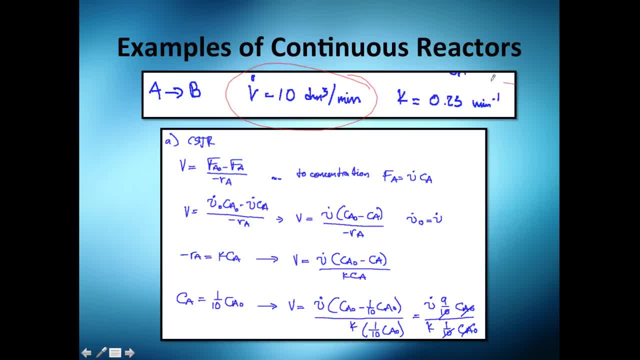 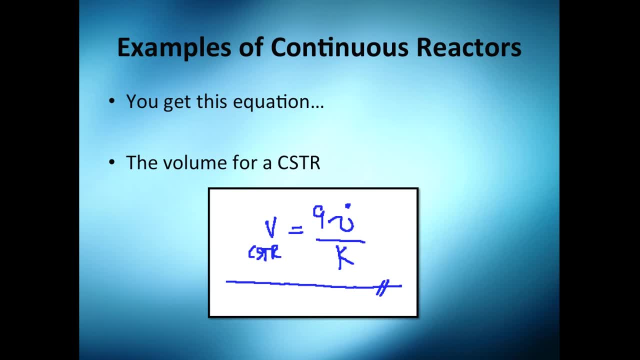 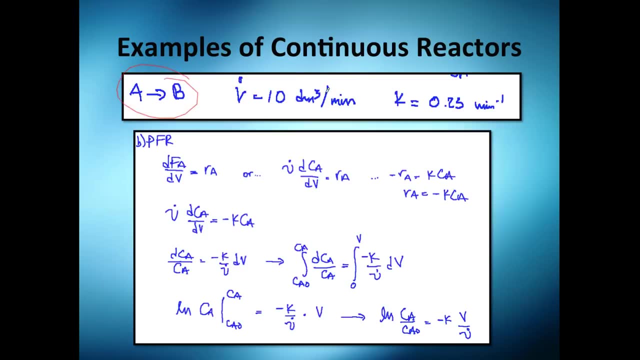 is the only data that we get: the volumetric flow rate and the constant. what a coincidence. okay, before calculating the volume, I want to calculate that of PFR. so I got the same data here, this equation, I got this volumetric flow rate. 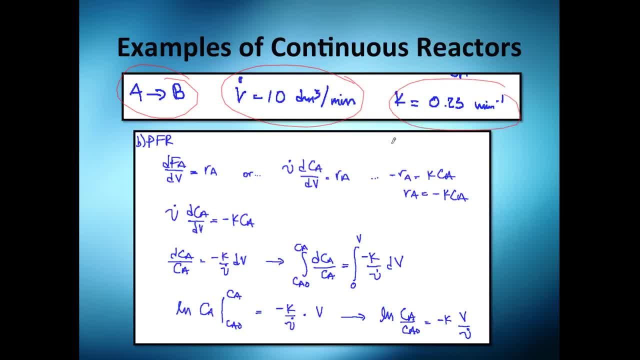 and this k exactly the same, because that is of the reaction, has nothing to do with my reactor. so let's model the plug flow reactor. remember, I'm going to draw you a diagram, so you are not. at last, you got an inlet, you got an outlet and the reaction happens here. 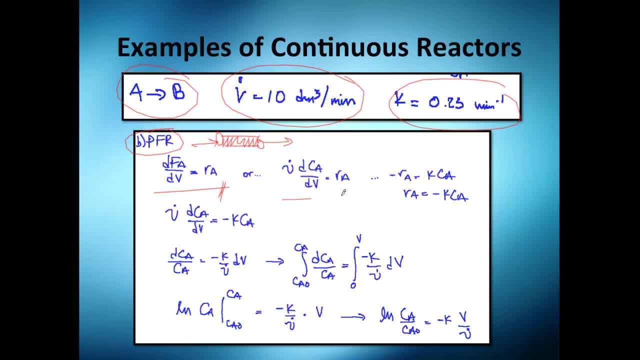 my design equation is this one or this one if you go directly to the substituted equation, which I will recommend you to do. so we got this equation. now we cannot go further because we need to substitute this value here. so I know that the rate of reaction 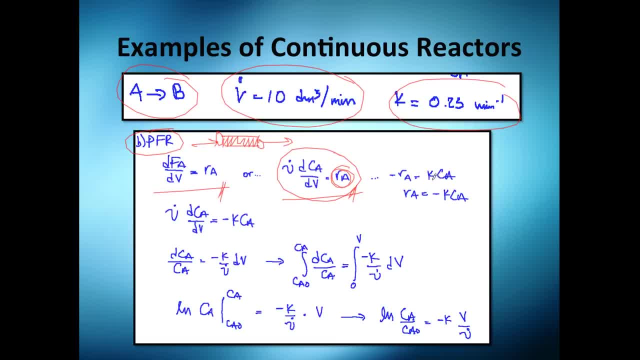 which is minus RA, equals the constant times the concentration. but I don't need negative, I need positive because I got it here positive, so I just change this negative here. okay, I substitute this data here, which is this one here: this stays the same: volumetric flow rate times the derivative as concentration with respect to volume. 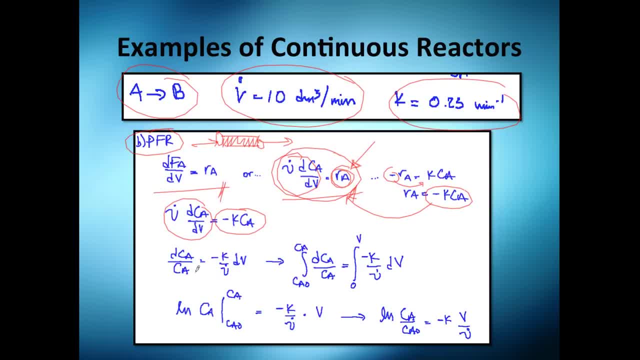 and, yeah, I will start doing my differential equation. I take out here my concentration because there is the derivative and the volume goes here constant and volumetric flow rate is once again a constant. so let us integrate from initial concentration to final concentration. is the derivative of concentration divided by concentration itself? 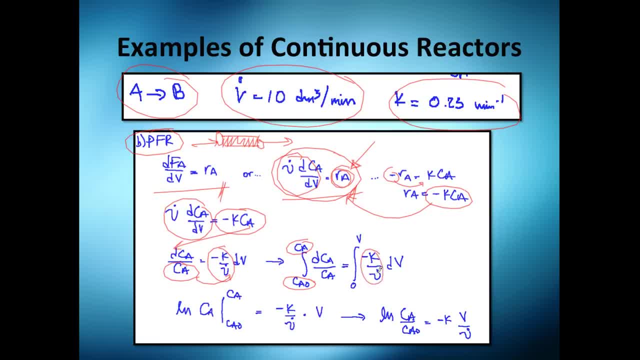 now from zero to volume, and this is a constant. so you will probably know that this beautiful integral is volume. so this is mathematics. the integral of one over C is natural logarithm of concentration. we need to evaluate it at final and initial and this is a value. and once again, I told you this was volume. 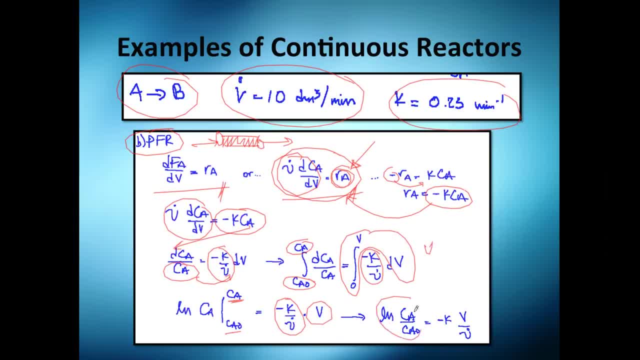 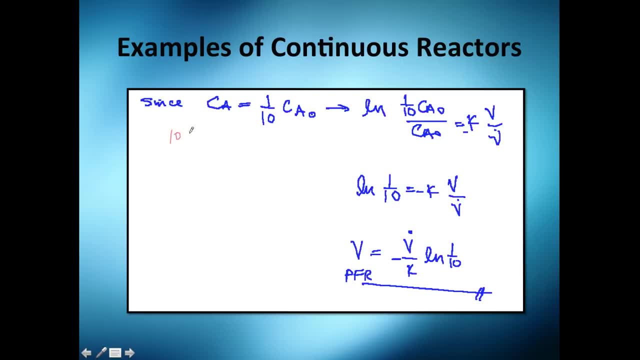 so I got this integral as volume. I evaluate this and I get this. so let me keep doing some math. once again, don't forget that they are asking us to do the 10%. so one tenth of the initial concentration is my final concentration. so this is my final concentration divided. 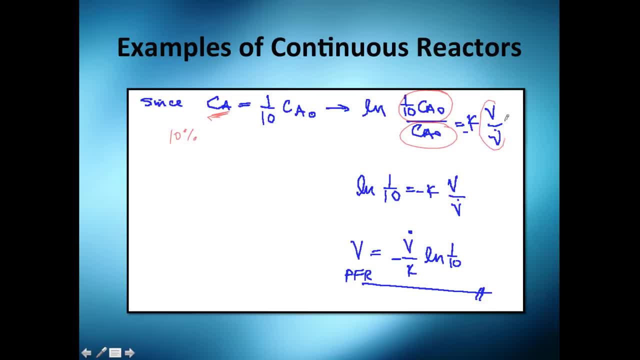 by initial concentration. and, yeah, this is constant. this constant, I got this value, which is actually a number if you check it in the calculator. this constant, yes, I have it. and this volumetric flow rate, I have it, so I can find volume. actually, let me find value: the volume use multiply volumetric flow rate. 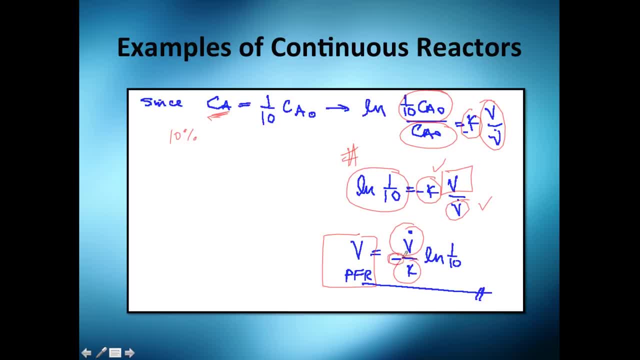 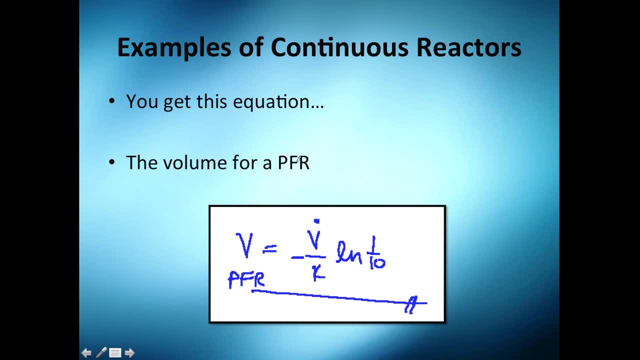 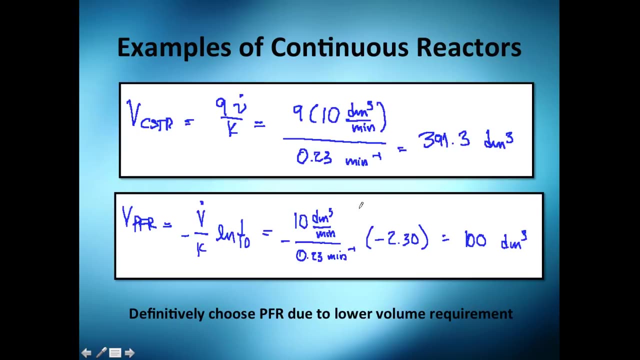 divided by the constant they gave us. don't forget this negative sign times the natural logarithm of 1- 10th. so once again you get this equation, which is the volume for a PFR reactor. now let me just once again check the equations I got. 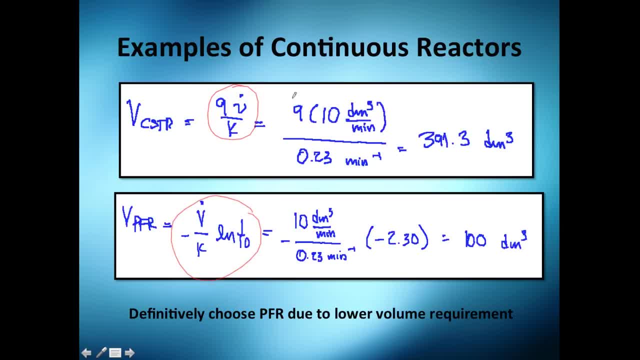 from my mathematical development. I substitute data: 9 times 10 cubic decimeters divided by minutes. all this is divided by this constant, which is 0.23 minutes to the minus 1. so thank God I got it. and now let's go back to the calculator and let's see what happens. 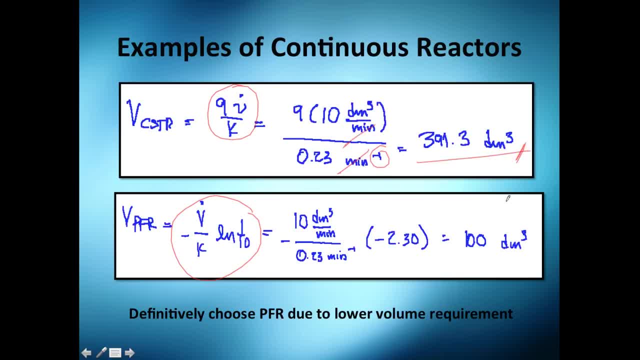 I can cancel this minute and minute and my solution and ops being cubic decimeters 391.3, which let's say 390 liters. now let's go to the plug. flow reactor substitute data. my volumetric flow rate is 10 cubic decimeters divided by minutes. then we got this K, which is 0.23 minutes to the minus 1 once. 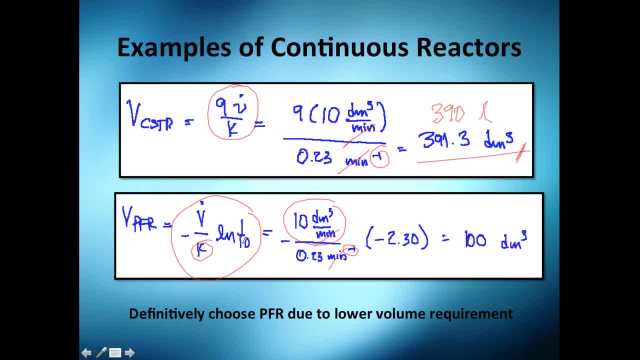 again. we will be able to take out those minutes and the natural logarithm of 1: 10th is minus 2.3, so 10 times that divided by this. once again, this is no coincidence- it goes out 2.3 and this 0.23, and then you got 100 cubic. 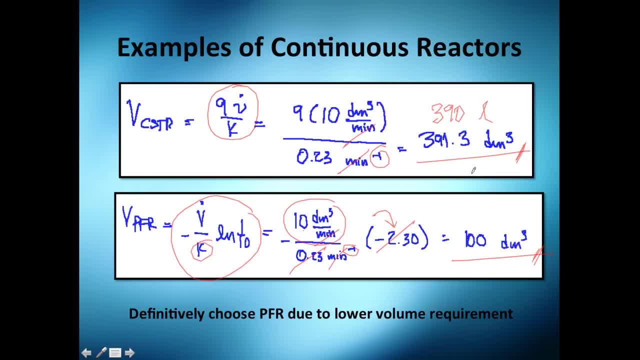 decimeters, which is almost 4 times less as our other reactor. so if you ask me right now I have no clue of what is the actual situation. I will say I will prefer the PFR. first, because it's less volume. second, less volume implies less cost of operation. third, it implies also less cost of investment. fourth, it's 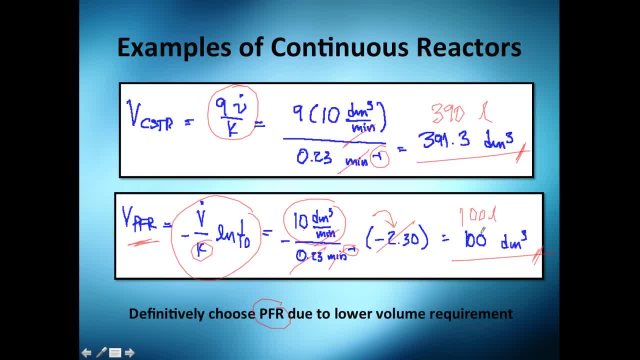 easier to operate in lower quantities than higher quantities. and also, yeah, essentially those are my reasons. of course, if your boss tells you I got a new, brand new reactor of 400 liters and it's already there and you have no money to invest, well, of course you will choose this one. but if you are starting from, 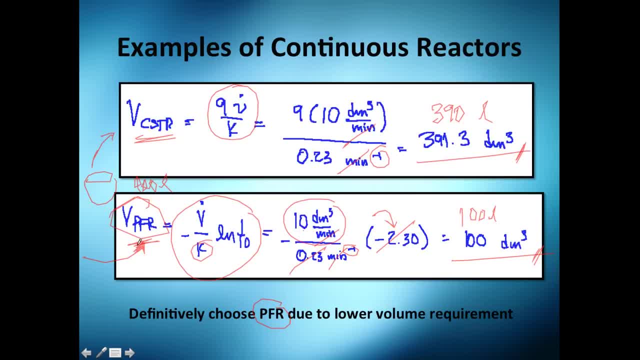 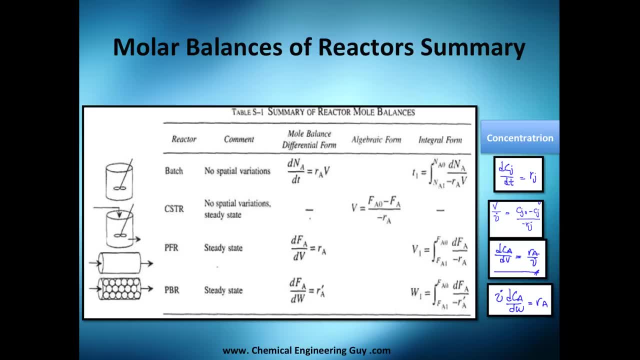 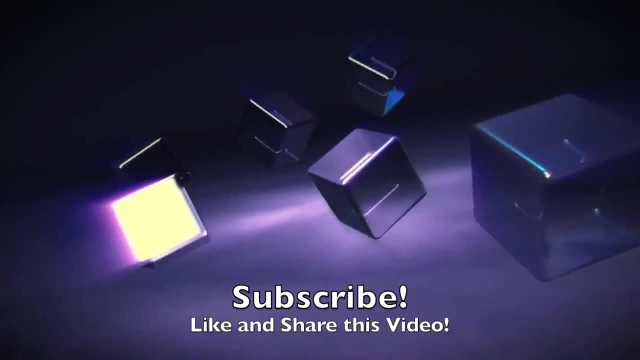 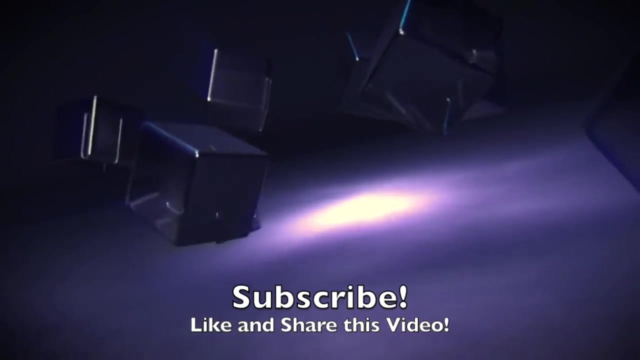 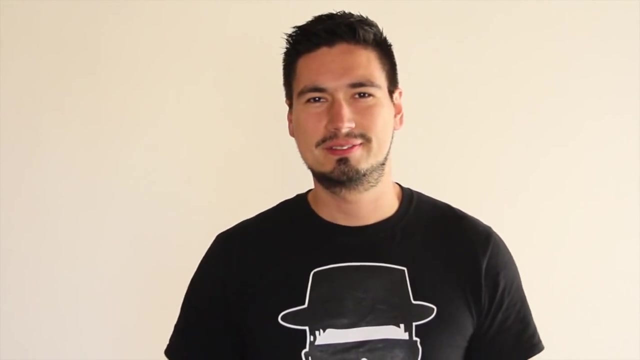 nothing. of course, this is the best decision, so that was my example. hopefully you like it. I think you will like more these tables, so keep watching, because I'm going to explain you how we got this table. what's up, guys, it's me chemical engineering guy. so if you like the video,